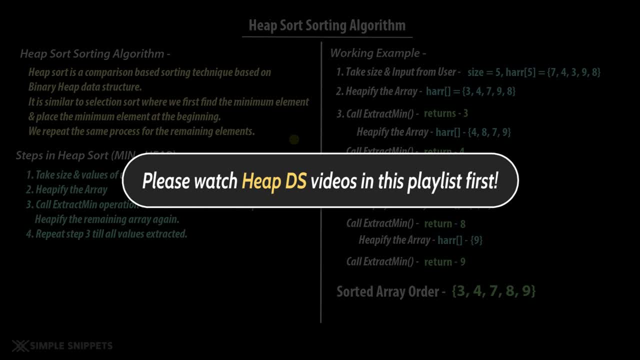 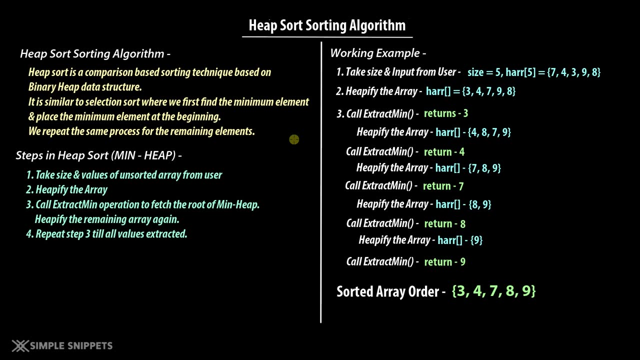 of heap data structure in previous video tutorials of this DSA playlist. So if you're someone who's new on this channel, who's not seen the entire DSA playlist, please check out this playlist and cover the heap topic, the main heap that we've discussed in detail with 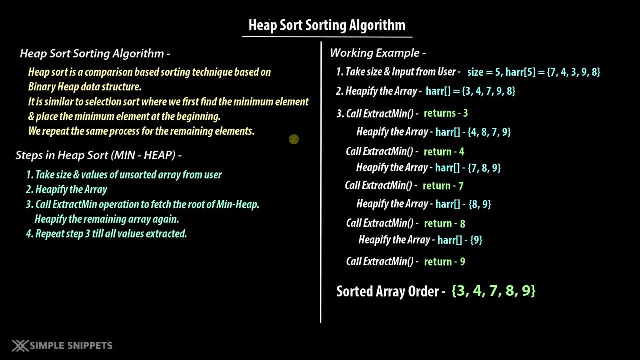 theory and with all the operations. We've also implemented all those operations in the form of C++ programming, especially the extract, main and heapify operations. If you don't understand those operations then understanding heap sort is going to be a little difficult, because heap sort is pretty much based on those two operations. So make. 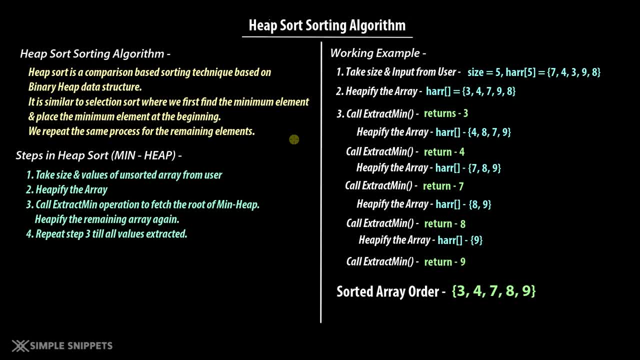 sure you watch those videos And if you've already seen that, you're good to go. things are going to be very easy in heap sort sorting algorithm. And with that disclaimer and with that introduction, let's start off with heap sort sorting algorithm. 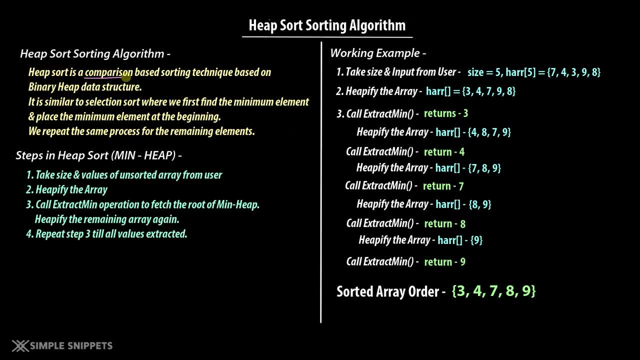 So a quick theory about heap sort. heap sort is nothing but a comparison based sort which is based on binary heap data structure, And it is similar to selection sort, where we first find the minimum element and place the minimum element at the beginning And we repeat the. 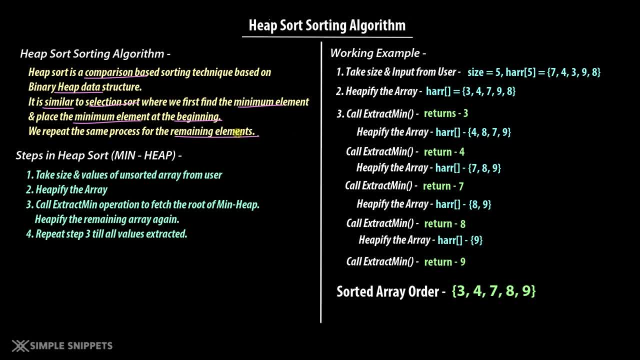 same process for the remaining elements. So it's similar to selection sort And because heap has a property that either the minimum value or the maximum value is always going to be at the root position, depending upon whether it is a min heap or max heap, that 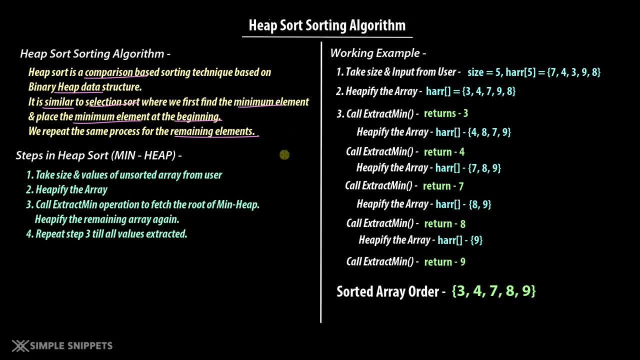 property is going to be utilized in heap sort. So in previous tutorials we've discussed- we've discussed that heap sort is a property that is going to be used in heap sort. So in previous tutorials we've discussed that heap sort is going to be used in heap sort. 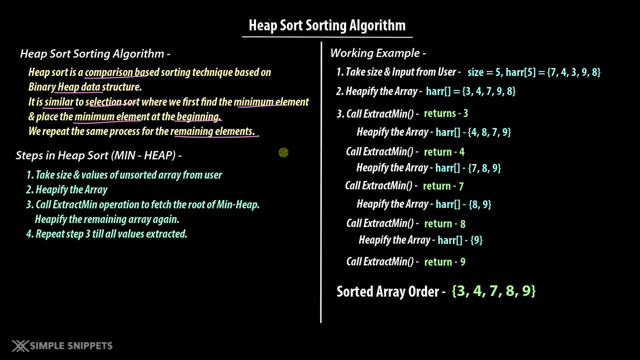 So in previous tutorials we've implemented min heap, So we're going to use min heap over here also. And in min heap, remember, we have the property that the minimum value will always be at the root level, right. And what do we do in a sorting technique? we basically arrange. 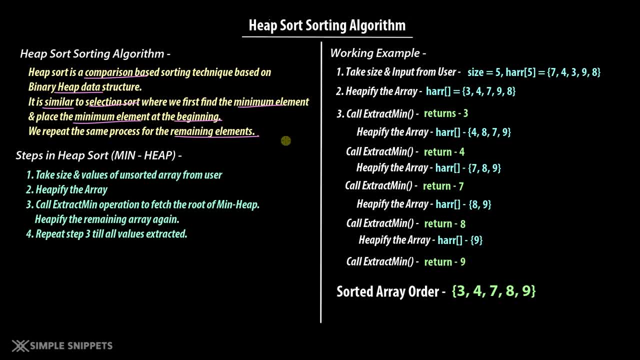 all the values in an array or in a list in ascending or descending order, And in our case we're going to use the ascending order. So we already have the basic logic formed over here. we know that in a min heap the minimum value is at the root level And we 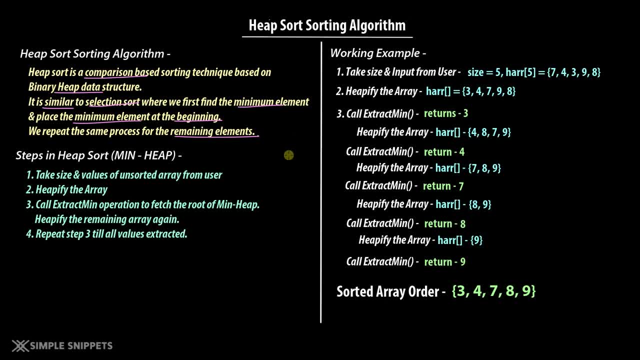 want to do sort Sorting, which means that we want to go from ascending to descending order. So the steps in heap sort go as follows: First we take the size and values of the unsorted array from the user. then we heapify that array. Heapify means creating a min heap or max heap. 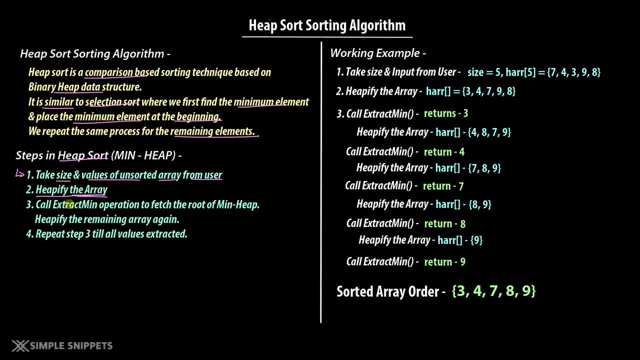 from a given array. So when you take the inputs from the user they will not be in a proper min heap format, right? When I say min heap format it means that min heap has a principle that for a particular node, it's children. 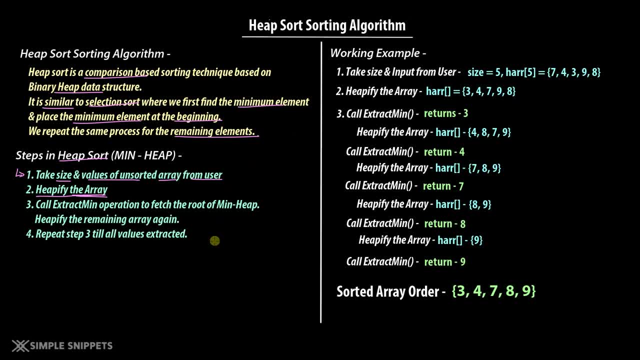 Children should be larger than that particular value. So let me just draw a quick example of min heap. So this right here is a binary min heap, because the minimum value is at the root level And both its children are larger. It doesn't matter how they are arranged. 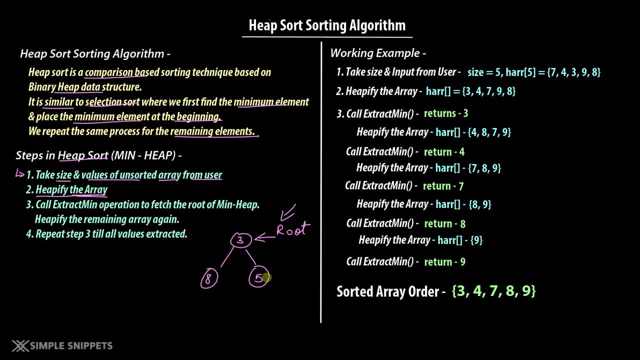 right, So you don't have to be arranging five at the left and eight at the right In min heap. the only concept is for every node, its children should be larger than that particular value. So if I have over here 9 and if I have over here 11 or 10, then this is valid For five. 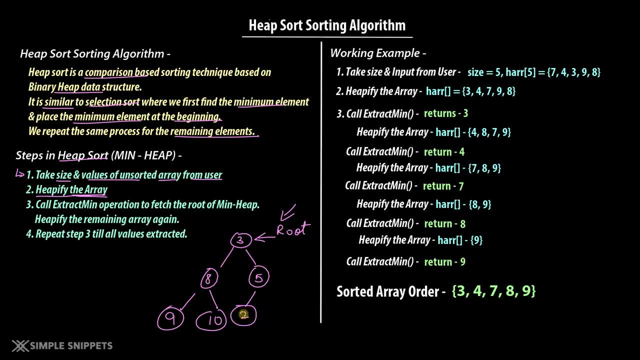 if I have two over here, then this is invalid because the root is three and two is smaller than three. So ultimately we have to bring two at this level. So this is one step in heapifying the process. or when you insert a new node, you have to get it back to its 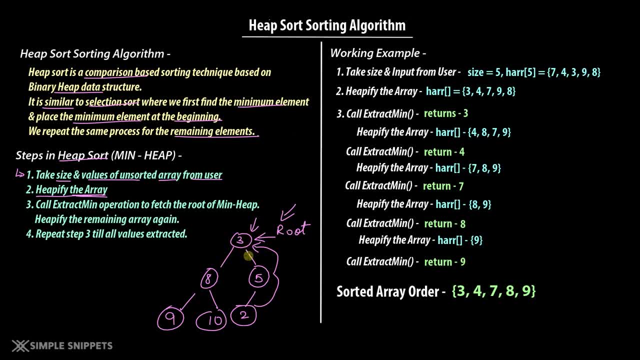 appropriate position to you know. follow the principles of min heap. Now, similarly, for max heap, the law will be exactly opposite, That is, the maximum value has to be at the top. Okay, But now, since we're dealing with min heap, let's talk about min heap only. But the concept 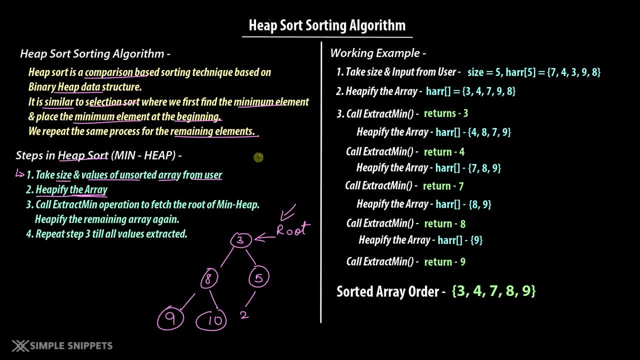 here is very clear: We are going to use this property of min heap. So we know that at the topmost value, or at the topmost root level, we have the minimum value. So once we heapify the array we will get something like this, And then we will call extract min operation. 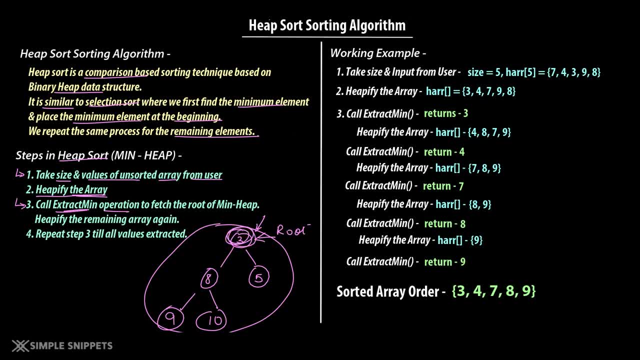 which will fetch us this root node and completely remove it off. So three will be printed And then we will again heapify the remaining array. So again some minimum value will come over here. Then we will again call extract min. So step four is basically repeat step three till all values. 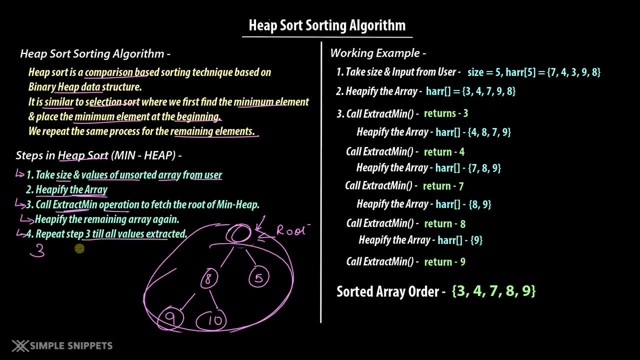 are extracted. So every time we extract a value, a minimum value will be extracted and it will be printed. So ultimately, we will get all the values in ascending order. And just to give you an example, this is how the working example would be. So, taking the size, 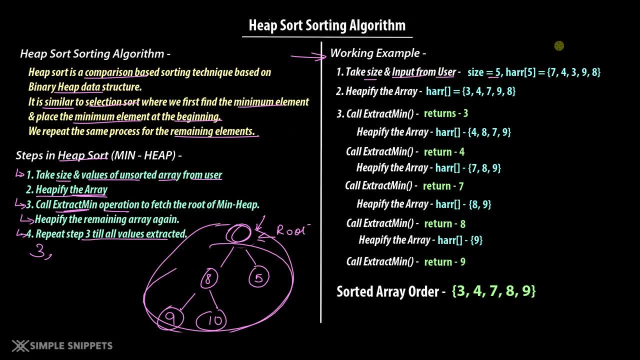 and input from the user. let's say the size is five. let's say the user enters this array in any order. So you can see this is not in any sorted order right, Seven, four, three, nine, eight. It is not in ascending or descending order. Our goal is using this heap sort to 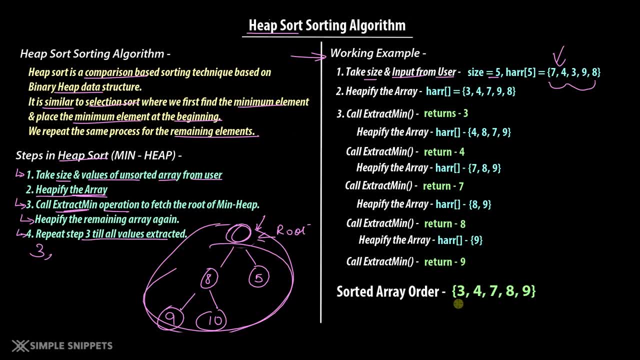 sort this. So the sorted value, that the output that we want, is three, four, seven, eight, nine. this is in proper ascending order, right? So this is what we want. So first thing we do is we take the size and input from the user, then we 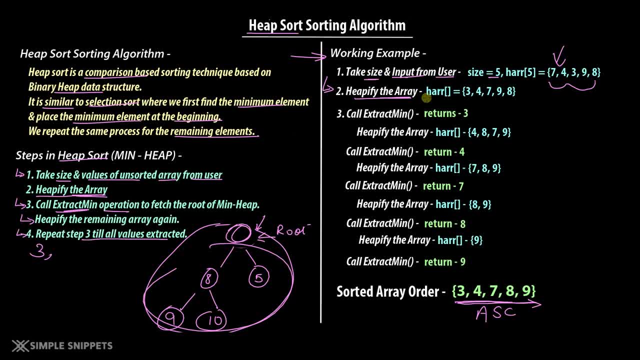 heapify the array. so when we heapify the array, we are basically creating a min heap, and the min heap would look something like this: 3, 4, 7, 9 and 8. okay, this is how structurally or visually, the min heap would look like. now, remember, we are implementing heap data structure using 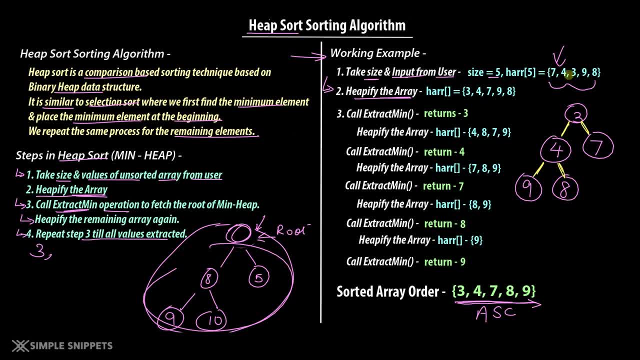 array, right? so even though the values are stored in the array, technically they are operating like a min heap, so visually you can represent them like this also, correct? okay, moving forward. the next step is extract min. so when you extract min, what do you get? you get the root value, which is 3. so 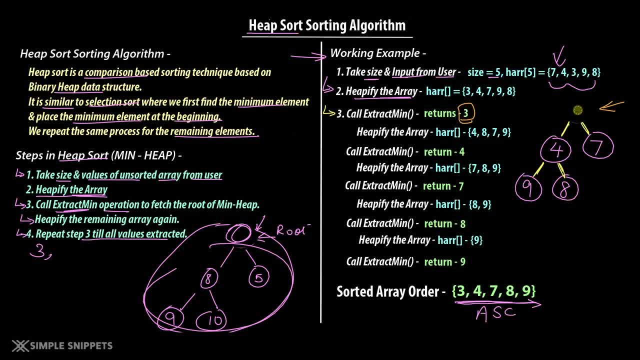 you can see 3 is printed. so once you remove this, the next step is you heapify the array again, and now you are left with 4, 8, 7, 9, so recreating the heap with the remaining values. so this is how the heap would look like once you return 3. 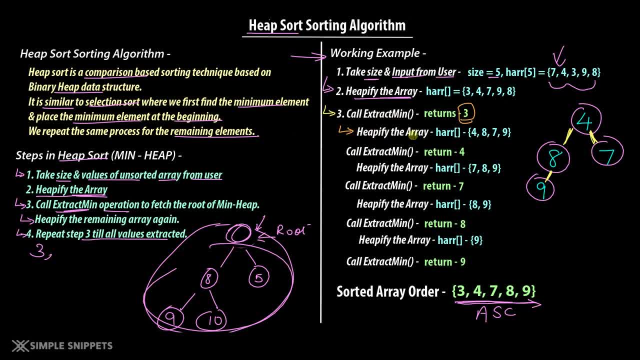 3, that is once you call the first extract min and after you perform the heapify. so 4, 8, 7, 9 is left. then again you will call extract min. this time you will get the top of the root, which is 4. so you got 3 and 4. you can see our ascending order is being created. so once you extract this, 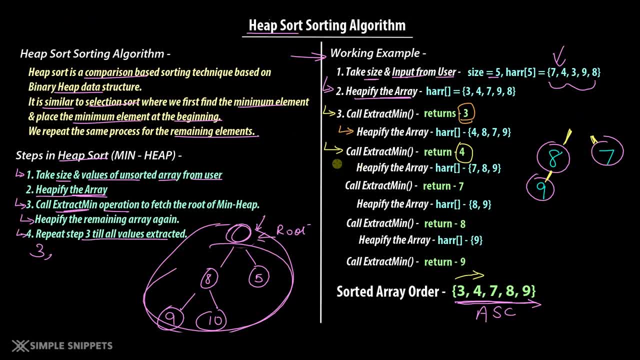 this will also be removed and then again you can see you have to do heapify. so after heapifying again, you will be remained with 7, 8, 9. so this is how the heap would look like when you are left with 7, 8, 9 and when you do the heapify. 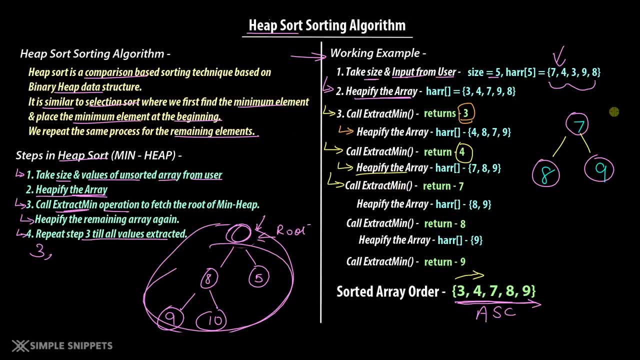 then again you will say: call extract min, so you will get the minimum value which is at the top root level, which is 7 this time. so 7 is printed. similarly, you will keep on heapifying and extracting till all the values are extracted, and the output is always going to be in ascending. 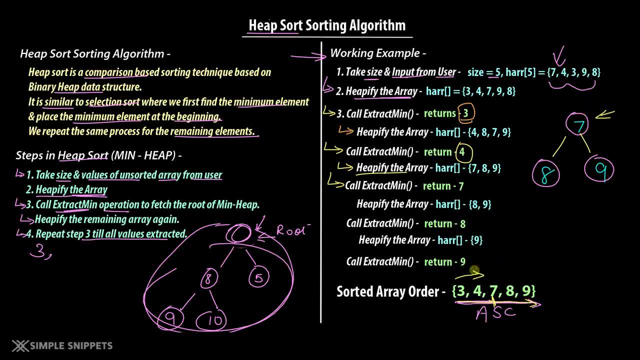 order, because every time you are extracting the minimum value, right, so 3, 4, 7, 8, 9 is being printed. so this is what is going to happen in heap sort, and this is the step by step working approach. but now we need to have a algorithmic way of converting this. you know, step by step process. 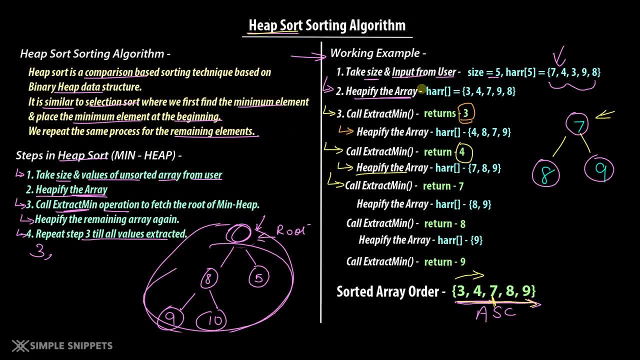 so we need to have a step by step pseudocode as well for all these english steps right, because ultimately we want to write a c++ program to implement heap sort. so by the end of this video we will also write a c++ program to implement heap sort. but let's first understand the pseudocode. 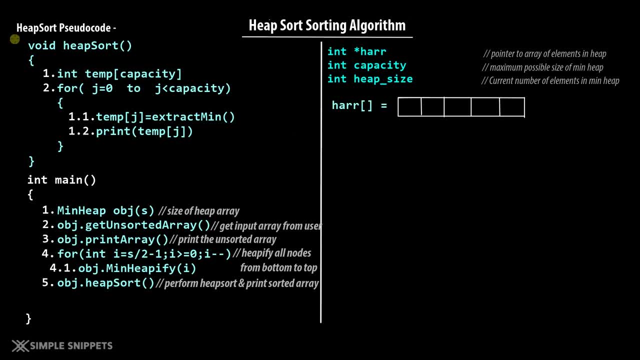 of heap sort sorting algorithm. okay, so over here is the heap sort sorting algorithm. it is pretty simple. it consists of only two things, that is, we have to extract min and every time you have to do the heapify. so extract min function is already there. i'll go step by step over here, but let's 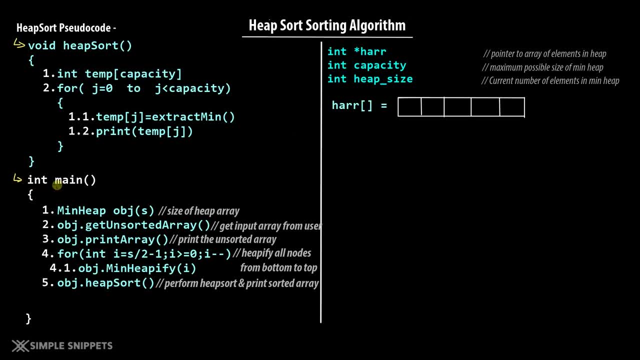 first take a look at what happens in the main function. so ultimately, we are going to write a c++ program, right, and the execution of c++ program starts from the main function. so in the main function, what we will do, we will create an object of min heap type. now again, for all of those who 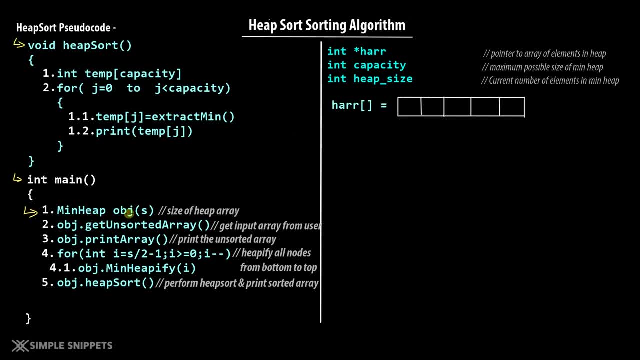 have not seen the previous videos on heap data structure. this is going to be a little difficult to understand, so please make sure you do that and we will see you in the next video, because we've already created the min heap class, which has all the you know data members, which are: 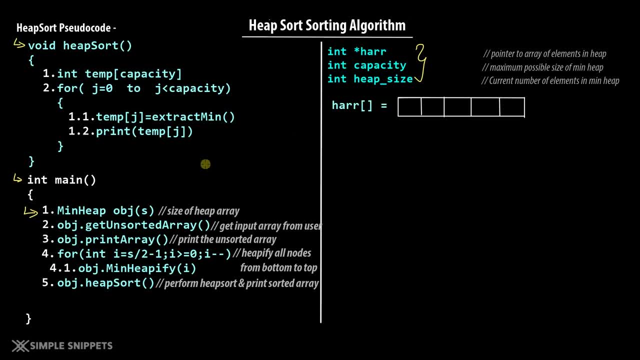 these three data members and also all the member functions like insertion, deletion, heapification, extraction, etc. etc. so here we will create a min heap, object obj, and we will take the size of the heap from the user. so s is nothing but the size of the heap. then we will say obj dot, get unsorted. 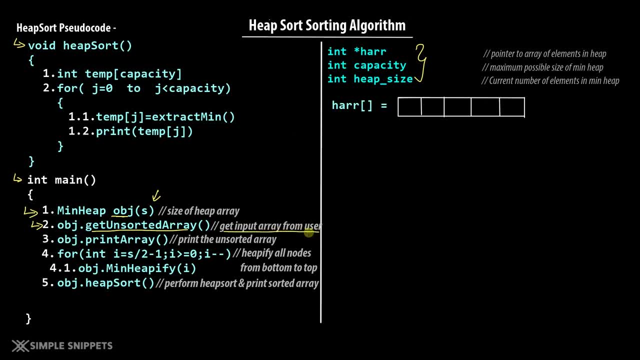 array. so basically we are taking the input array from the user. okay, so let's do this side by side by dry running this code. so let's say, the size s that you are going to enter is going to be equal to five. okay, so this size will be assigned as the capacity and 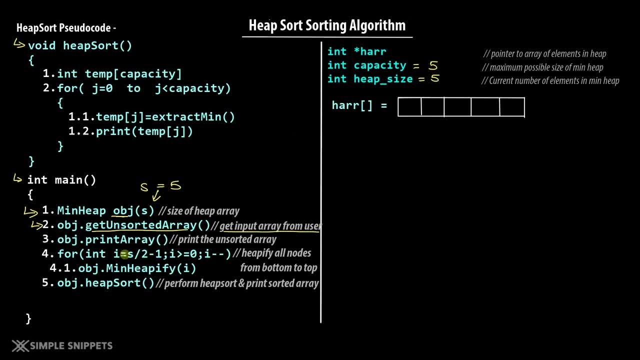 heap size both. that is because the user is going to enter five values, right? so at step two you are saying: get unsorted array. so basically nothing but take the input array from the user. so let's say the user enters some random five values, so let's note them down. 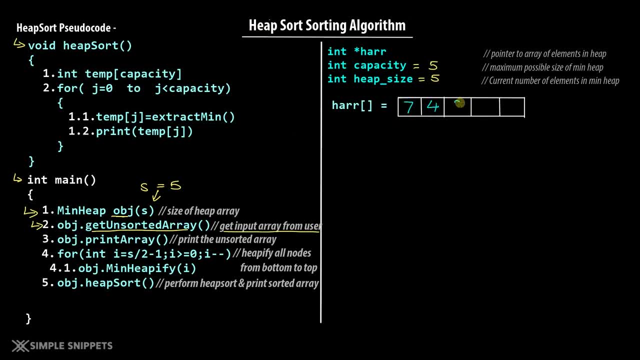 so let's say the user enters seven, four, three, nine, eight. okay, so this is a unsorted array. this is not yet a min heap, because this is not yet following all the principles of min heap, correct. step three is we simply print out the array. basically, we'll print this as it is, so i'm not. 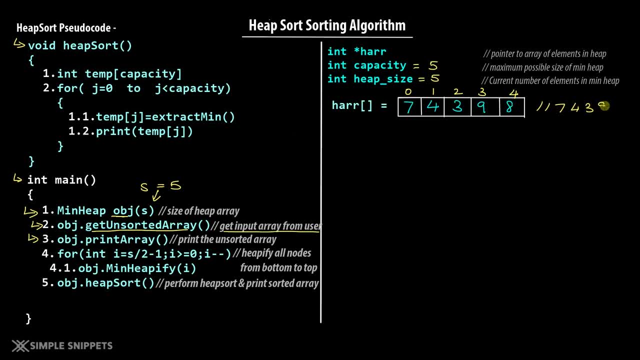 doing it over here. so seven, four, three, nine, eight will be printed. so before sorting you want to show. step four is, as i mentioned, you need to first heapify this array. when you heapify this array, the minimum value will come at the root level right, because this is a min heap. and then you 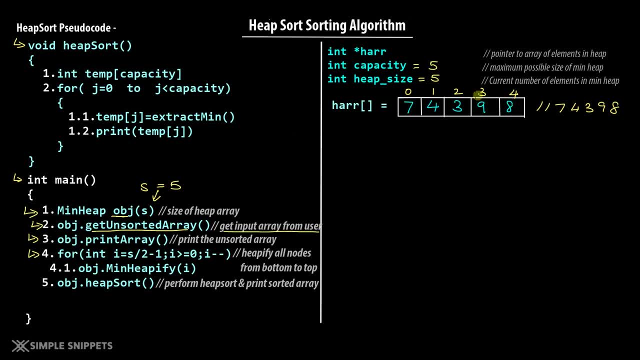 can do the extraction. so for the first time, when the values are all random, you have to heapify all the nodes and that is the reason why you have to run a for loop. so currently, if i draw a structure of binary tree of this array, the values that we will have is seven, four, three, nine, eight. 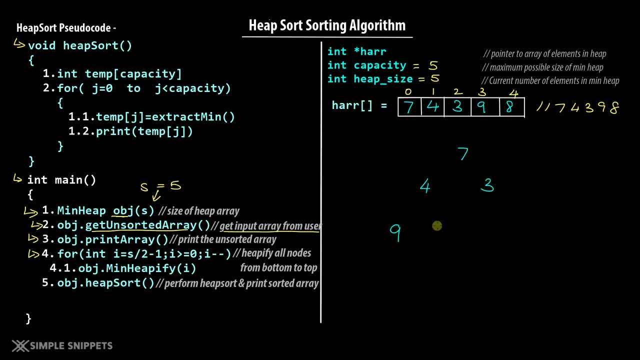 seven, four, three, nine, eight. that's how you assign the values, that is, the positional values of an array. for a min heap right, you go from top to bottom, from left to right. so right now, this is how the min heap is, and this is actually not a min heap right. you still have to heapify. 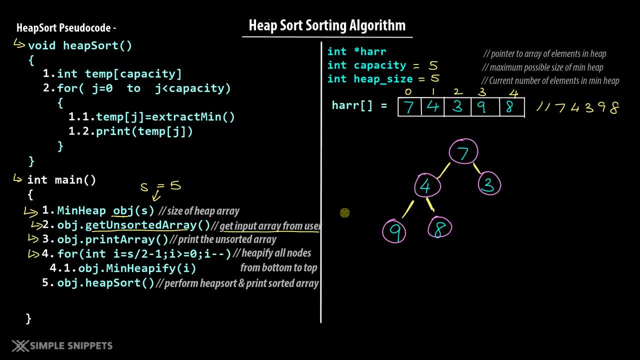 this correct. so now we have to heapify all the nodes, which means that we will have to start from the bottom and go to the top of the array, and then we will have to heapify all the nodes. the top, that means we'll have to start the heapification process from the leaf node level. 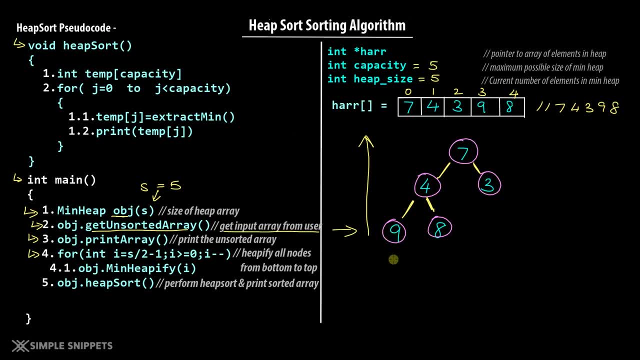 actually one level above the leaf node. that is because for this particular node, if you apply heapify, there is nothing below 9 and 8 right. so you don't have to apply heapify. this is already heapified. so you'll have to start the heapification process from one level above the root level. 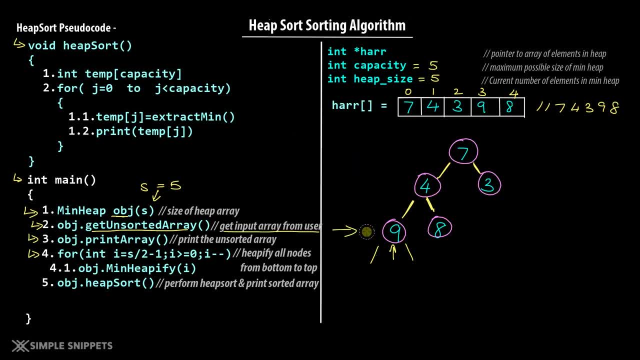 okay, always remember this: we have to start heapification from the bottom level to the top level and we have to exclude the leaf level. so this is why we will run a for loop. we will say: i is equal to s by 2 minus 1. s, as i mentioned, is nothing but 5, right? so i is going to be 5 by 2. 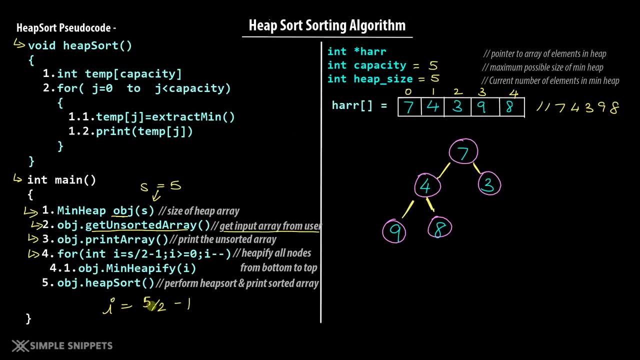 minus 1, so 5 by 2 is nothing but 2.5, and this is the integer. you will exclude the fractional part, so it will be 2. 2 minus 1 will be 1, so i will be nothing but 1. so you'll start from. i equals to 1. 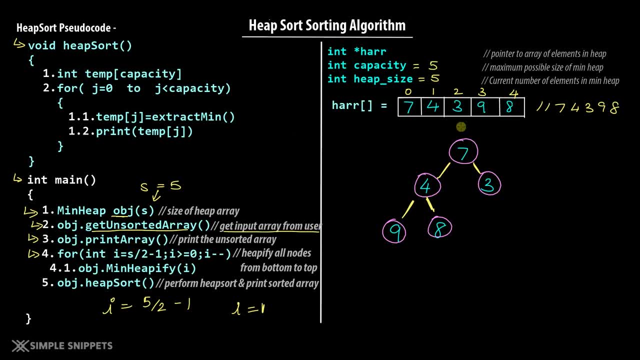 and you'll run till i is greater than equal to 0. so this is index position 0, 1, 2, 3 and 4. so we'll start from index position 1. right, we just calculated i equals to 1. let me write: i equals to. 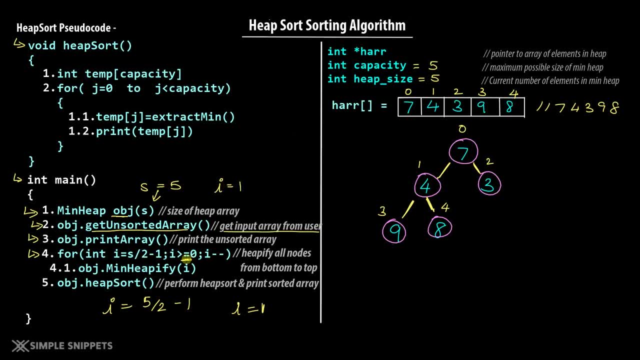 1 over here. is i greater than or equal to 0? yes, so we'll start hippification of this node, because you can see, this has two children and this is one level above the root level, correct? let's just say we had two more values. okay, let's assume we add two more values, which means that 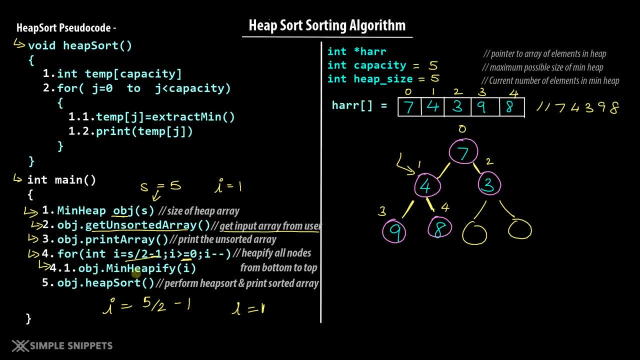 the total size is going to be 7, so then the formula would become 7 by 2, which is 3.5, which means 3, 3 minus 1 is 2.. so in that case we will start hippification from this node, because it 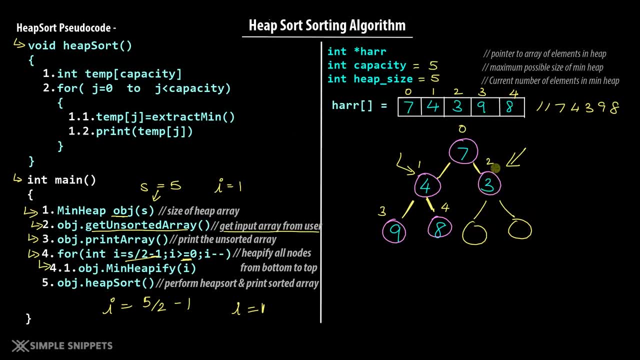 has two children, so you'll have to make the comparisons of which one is smaller and get it at the top correct. hippification is nothing but creating a heap from the existing tree values and remember the minimum value will always be at the top, so in case if there was one over here, 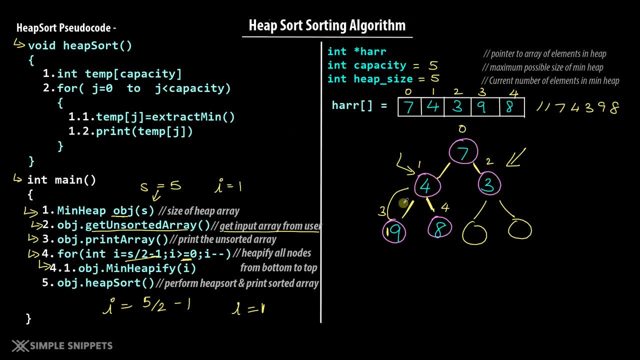 this node would have come at this place, correct? so that is what min heap is all about. so first time we'll call min heap on this particular node, because you're passing i. so min heapify is nothing but a function which we will create, which we have already actually created. 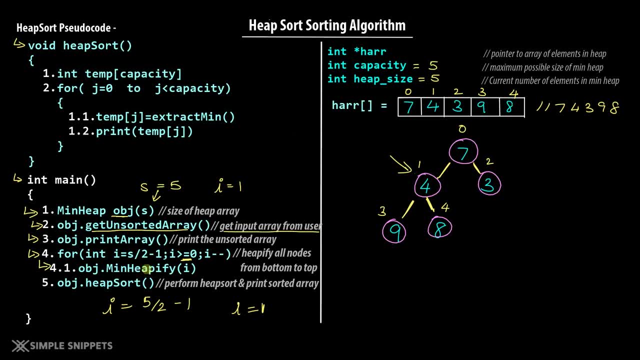 in previous tutorials. we are simply calling it over here. i'll show that function to you in a minute- and we are passing the index position i, which is nothing but a one. for the first time. this node will be heapified right now. there is no need to make any swapping over here. you can see. 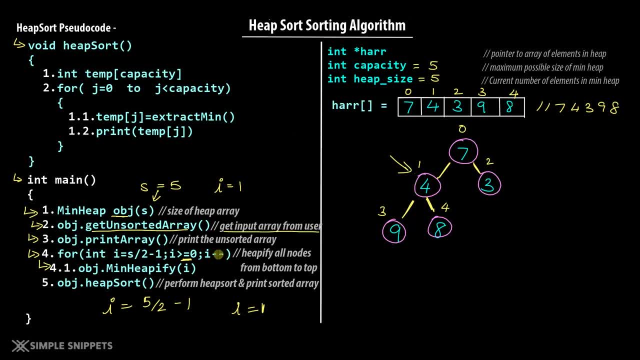 it is already heapified, then i will become minus minus, which means i will become zero. is 0 greater than equal to 0? yes, so now we will hipify this value. that is this node. so this root position 7 is definitely needs to be hippified, because 7 is not the minimum value. so ifification will take. 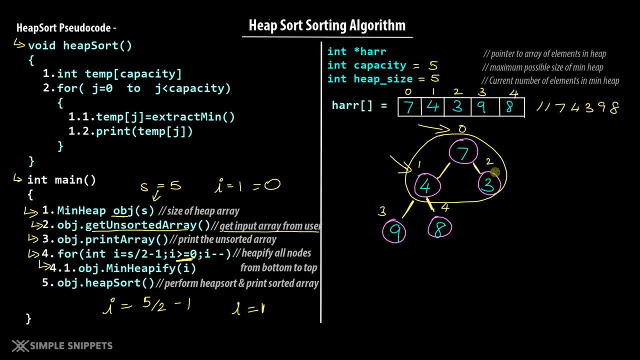 first these three nodes and compare which one is the smallest. so three is smallest, so three should come over here and seven will be swapped over here, correct? so ultimately we will get three over here, we'll get seven over here and in the array also. this will happen, correct? 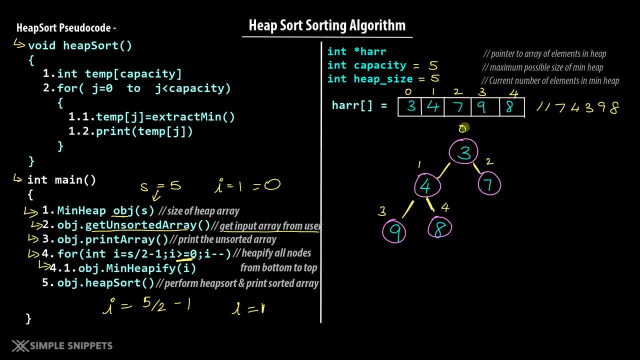 so three will come over here, seven will come over here, and now we have basically got our proper valid min heap. so this is a min heap, and then i will become minus, minus. i will become minus when this loop will break out, and now we can call heap sort. okay, so this is again our user defined. 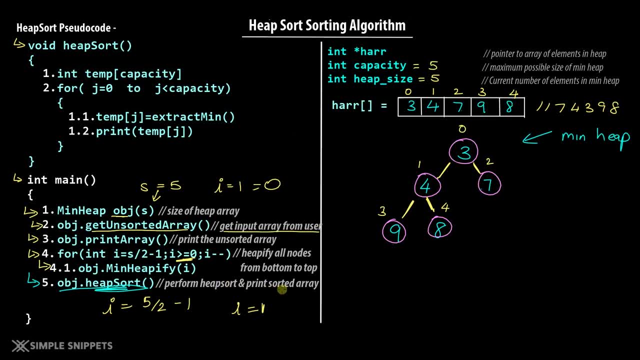 heap sort function. so this will perform the heap sort as well as print the sorted arrays. so basically, what it will do is these steps correct. so let's see what heap sort does. first we will create a temporary array with the same size, so capacity is five. so temporary array. 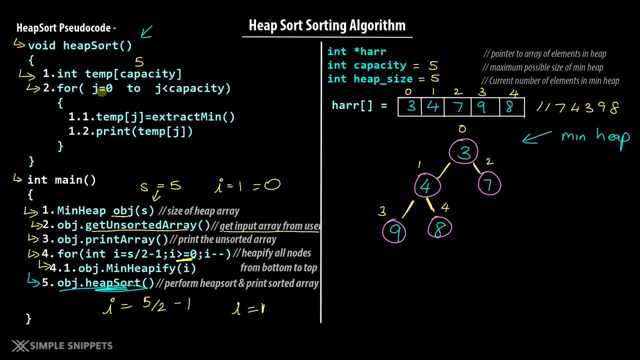 will also be of size five. next thing, we will run a loop. for this loop, we will run it from zero till five, which means we will run from zero, one, two, three and four, which means it will run five times correct, and in that, five times the only thing that we are going. 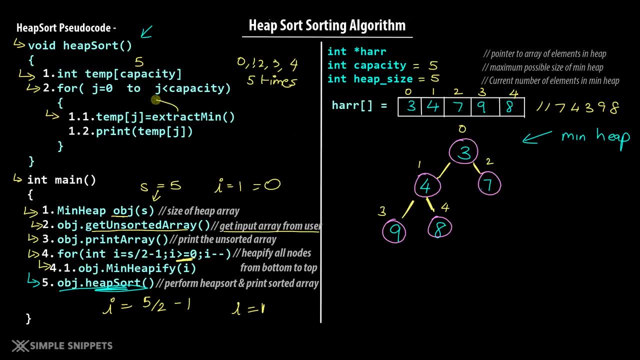 to do is we will say extract min, so minimum value first time will be three. it will be put at index position zero for the first time. then we will print out this value. you can also print it outside the for loop, but right now i'm just printing it over here. 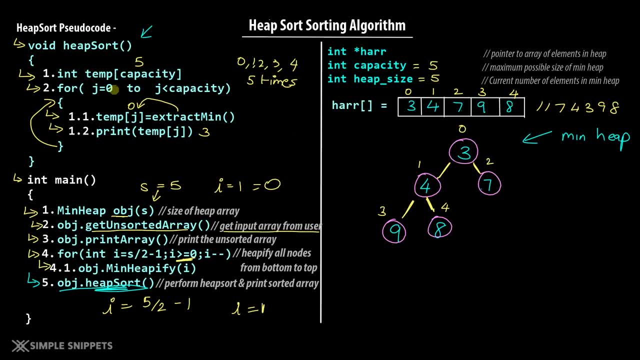 three will be printed first time. then you'll come at the start of the for loop. j will become one. j is less than capacity, capacity is five, right, so one is less than five. then you'll go inside. you will say: temp of one is equal to, again, extract min. now remember, when you call extract min. 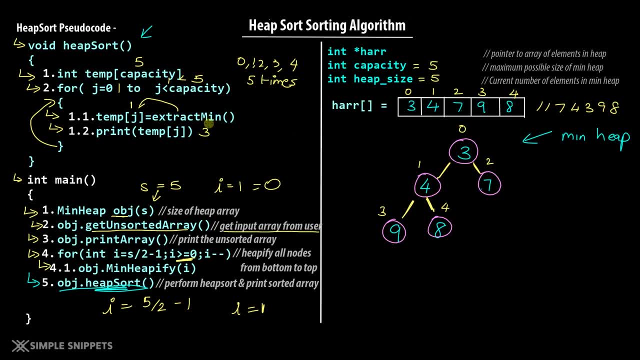 extract min is a function which already has heapify in it, so extractman will extract this value as well as heapify the array again, so you don't have to explicitly call heapify over here. so if you just want to see the pseudocode for extractman, let me just quickly show it to you. i have completely covered it step by step in. 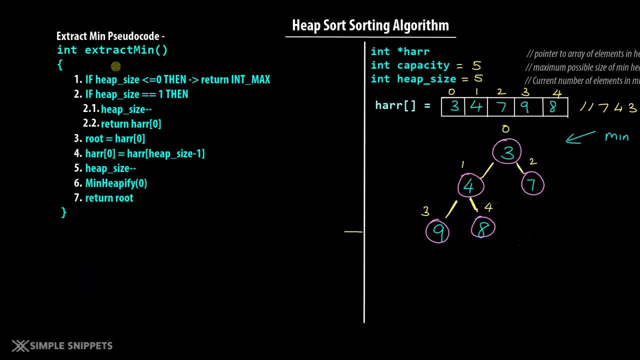 previous tutorial, so we will not go in depth over here. so this is the extractman pseudocode. if you want, you can take a screenshot and you can try run this step by step also again, for you know practice purpose. but coming back to our heap sort code, it's basically just this for. 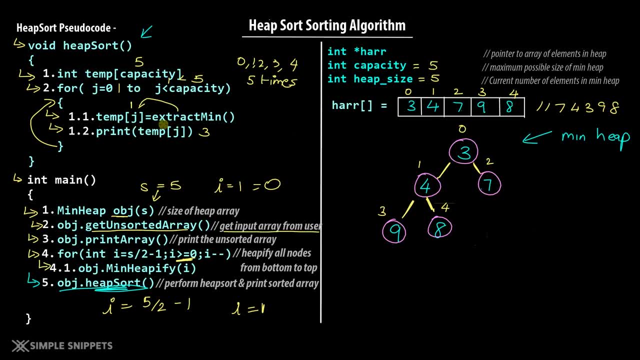 loop which will do the everything. that is because extractman is basically doing most of our work of extracting the minimum value and again heapifying the entire array, and then you simply have to print the values. so this is the entire heap sort. it is just few steps, but provided that you already have written. 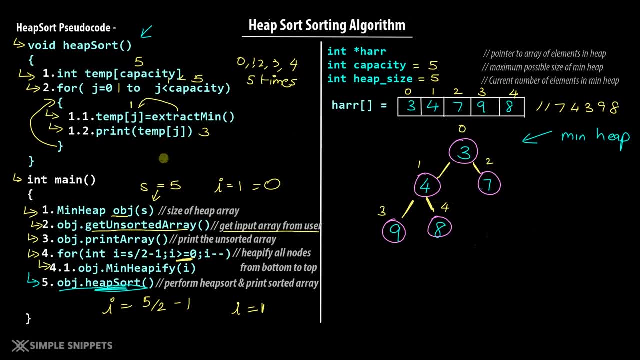 the code for extractman, as well as the heapification process and the initial steps, where you take the size of the array from the user and perform heapify. okay, so there is a little bit of initial processing, but the heap sort program is fairly easy. now let's jump to the c++ code, id and 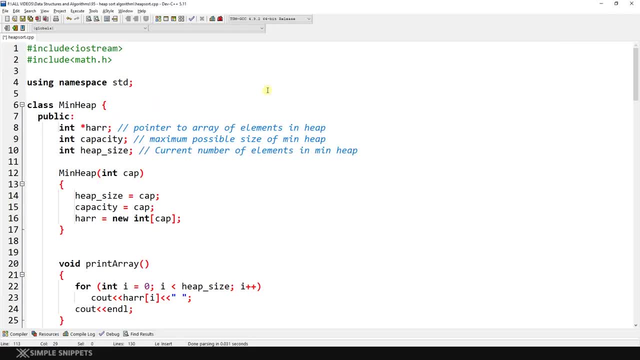 see the program in working okay. so, as you can see on the screen, we are in our c++ id, which is dac++id. we've already typed in quite a lot of code. this is all the code that we've been doing in the previous tutorials of. 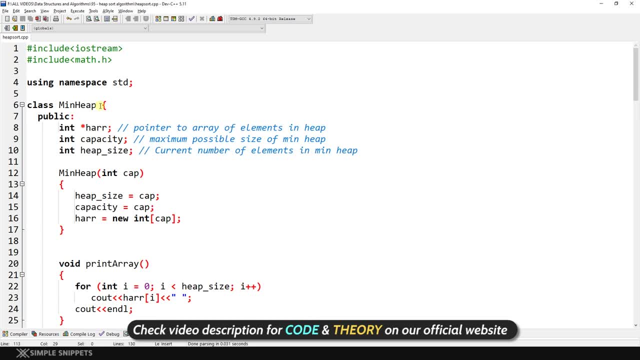 heap topic. so i have just used that same code over here. there is a small difference in the constructor, the parameterized constructor. here we make the heap size and capacity as same in the heap videos. this heap size initially is zero, but because of the heap size and capacity as set to zero 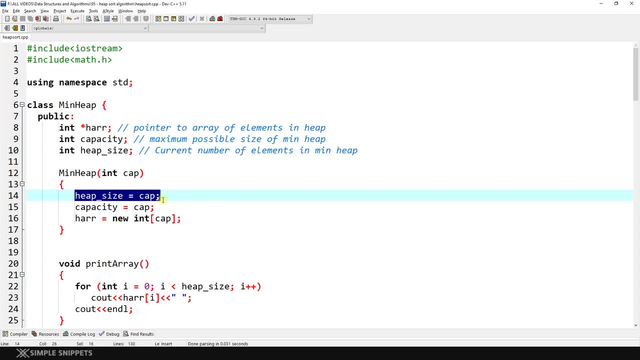 in our heap sort, we are going to take all the values from the user at runtime in one go. we are assuming that the heap size and capacity is the same. okay, so that's one small difference, but apart from that, everything else is taken directly from that code. and don't worry, guys, if you don't have. 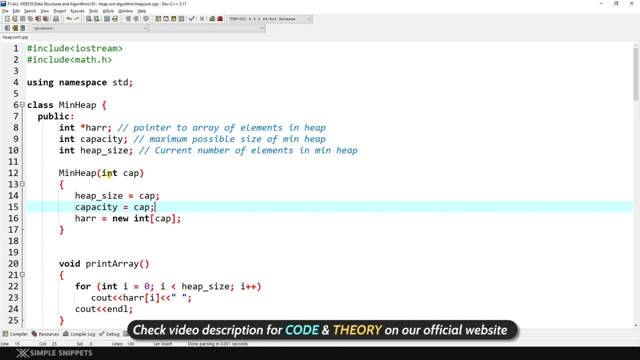 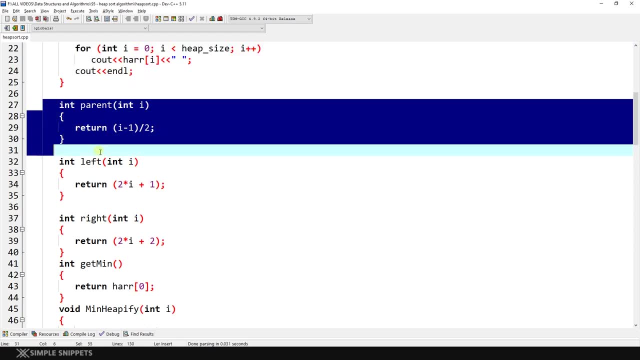 this code. i'm going to be sharing this code on our official website. you can see a link in the video description to get this code. so, coming down, we have the printing of array. we have the parent left right. get min functions- again, we've discussed all this in previous tutorials. then we have the 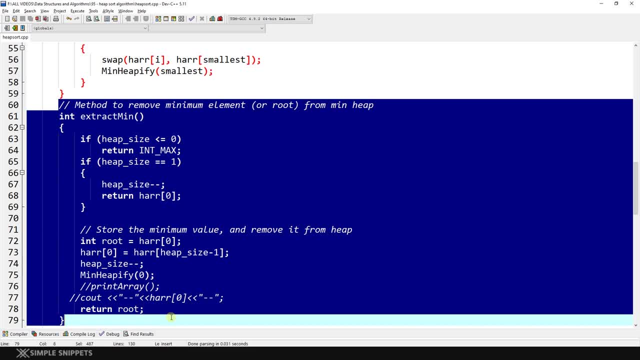 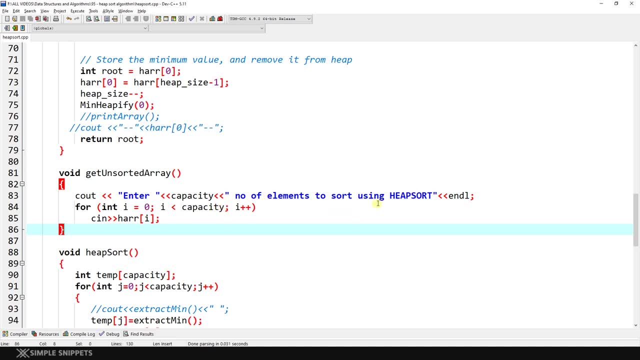 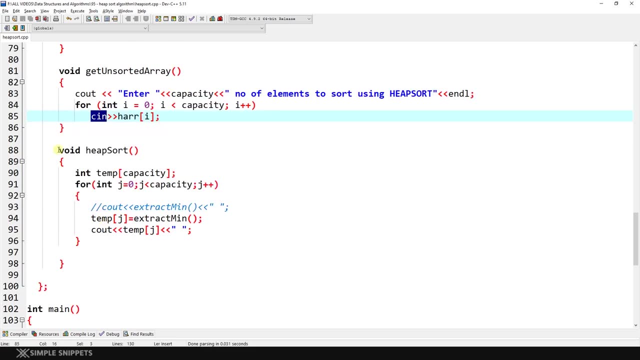 min heapify function and we have the extract min function. lastly, we have the get unsorted array wherein you know, we say, enter the capacity, that is the number of elements you want to sort, and then you take it from the user using cn. so this is where you take the input from the user. then 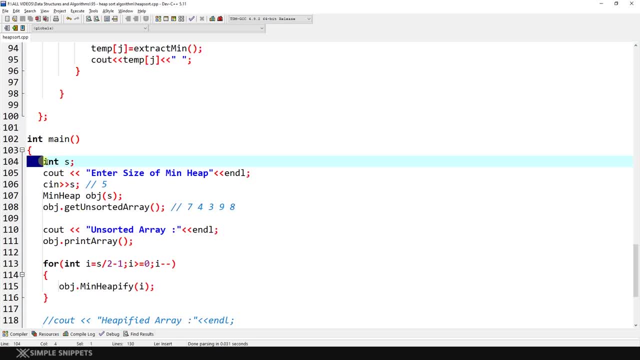 you perform heap sort. okay, so in the main function again you declare s, that is the size of the min heap. you take the size from the user by saying: enter the size of the min heap, then you create a min heap object. so min heap is nothing but this class that we've created on top over here. this. 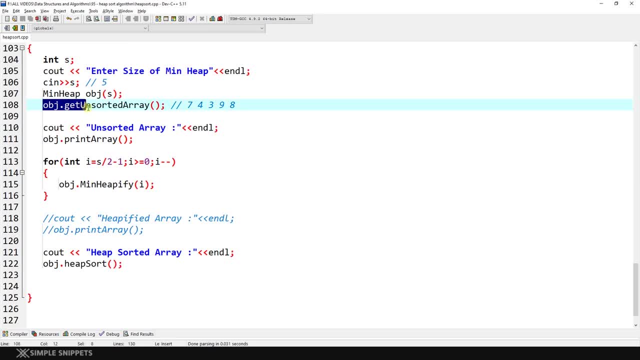 is the entire min heap class. so, coming down, you take the unsorted array from the user. let's say the user enters 7, 4, 3, 9, 8. that is the example that we just saw. you print out the unsorted array. then you perform min heapify on all the nodes. 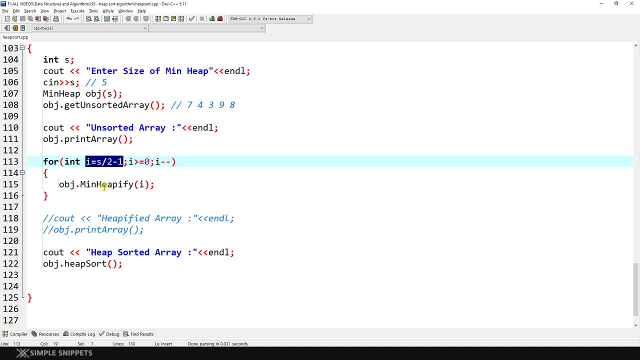 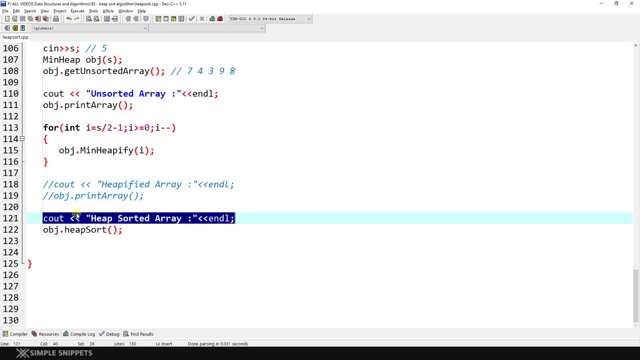 by using this formula, you can also perform min heapify on the leaf nodes. it's just that it is not necessary. but remember that you have to do the min heapification from bottom to top- okay, not top to bottom, it won't work like that. and lastly, you simply have to say heap, sorted array and call. 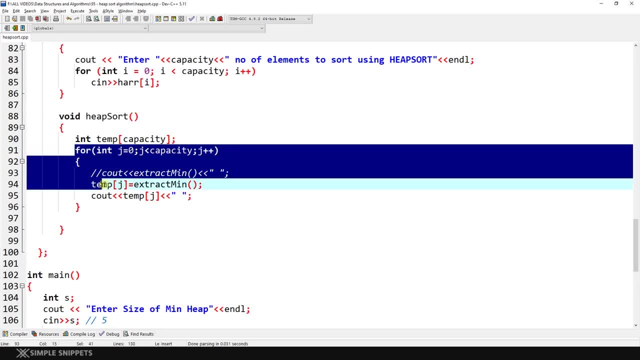 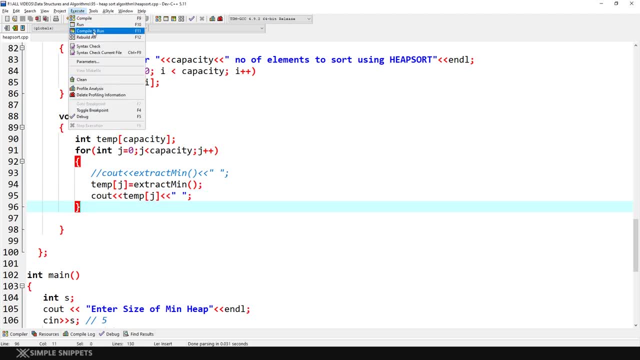 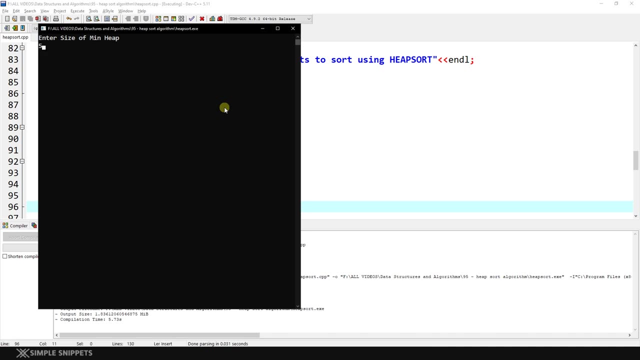 the heap sort, because in the heap sort function itself you're printing all the sorted values. right? this is where you're printing all the sorted values, so let's save this. let's go to execute, compile and run. let's see if this works. okay, so this program is working. let's enter the size of the min heap, let's say 5. let's enter the. 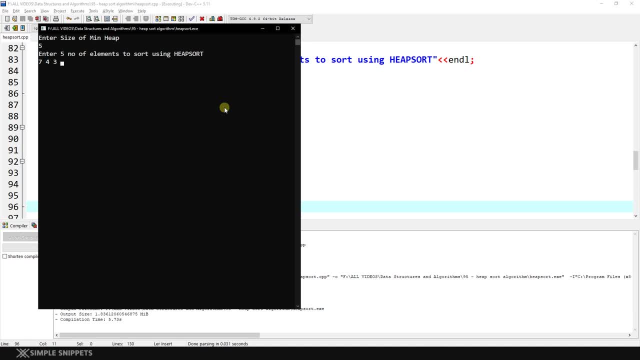 same values that we just ran: 7, 4, 3, 9 and 8. when you hit enter, you get the unsorted array, as it is 7, 4, 3, 9, 8, but the heap sorted array is 3, 4, 7, 8, 9, which is in proper ascending order, which means: 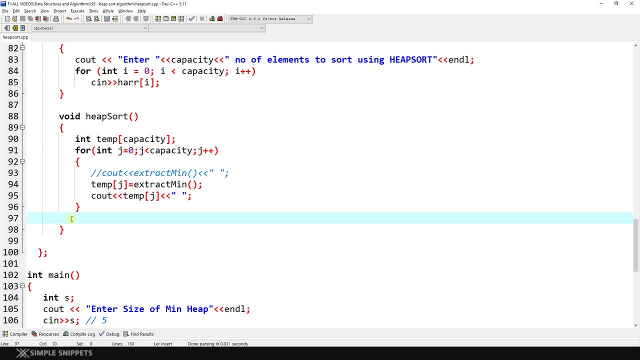 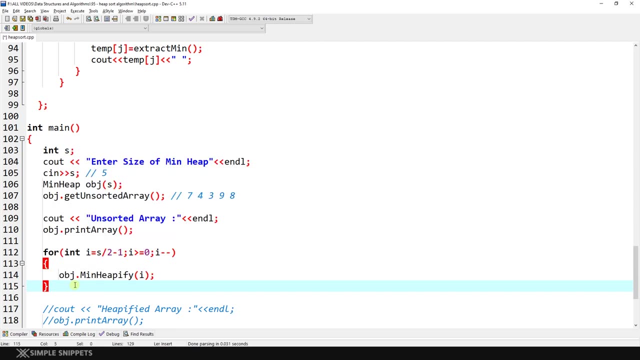 our heap sort is working perfectly fine now. if you're a beginner and first time watching this video, please type this code at least once. but you can still get it from the website. try it on your system. i'm pretty sure things will work perfectly fine. and this is where we've successfully understood and implemented the heap sort sorting.